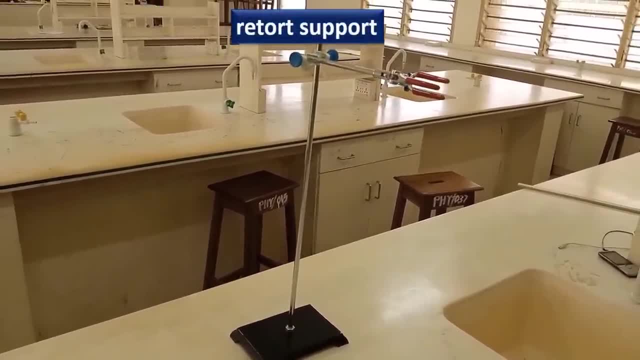 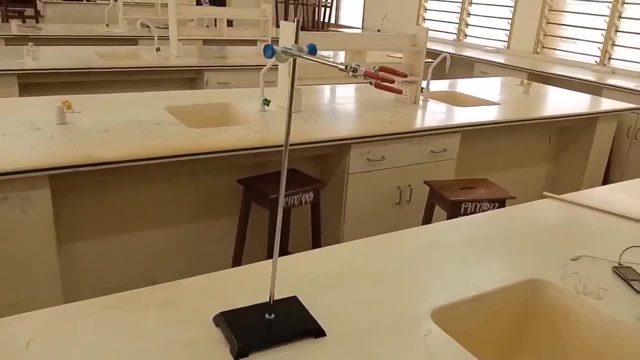 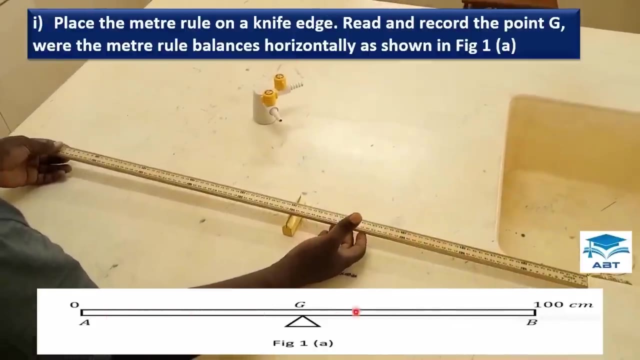 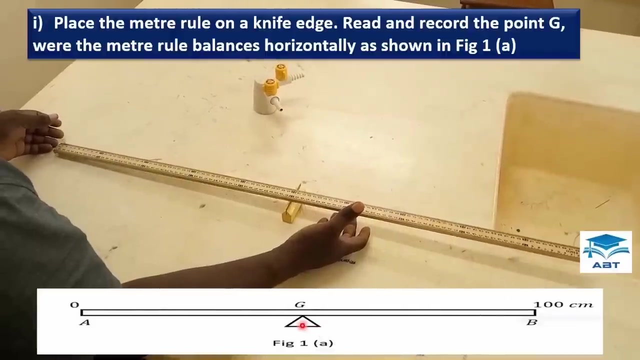 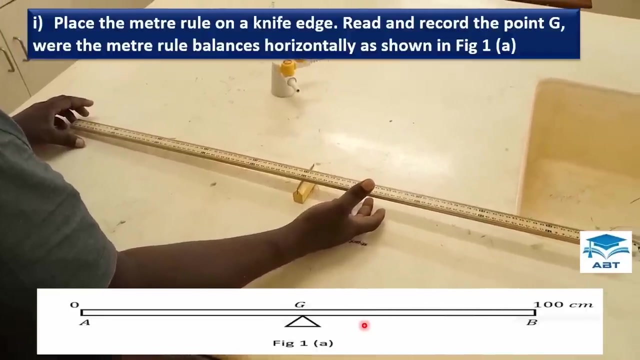 Retort support And other necessary apparatus. We are going to balance the meter rule horizontally on the knife edge, as shown in this diagram, and determine the point G where the meter rule balances horizontally. However, it won't do any good for their safety. 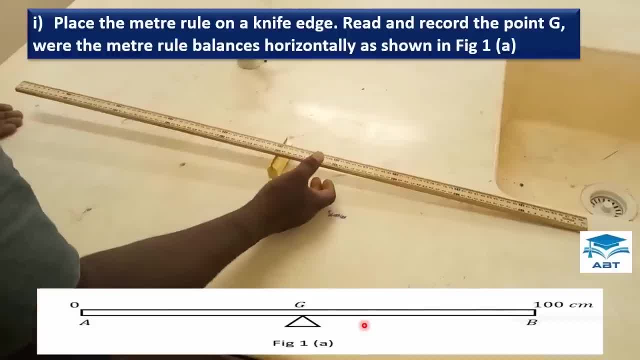 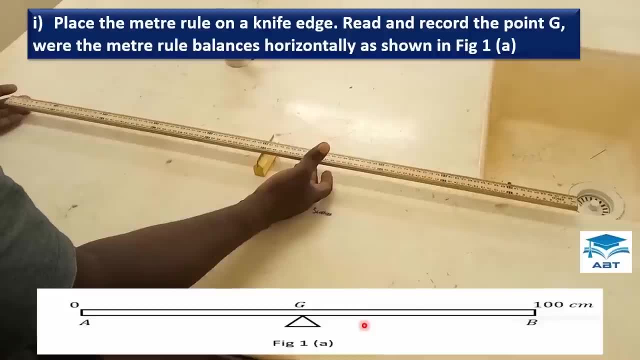 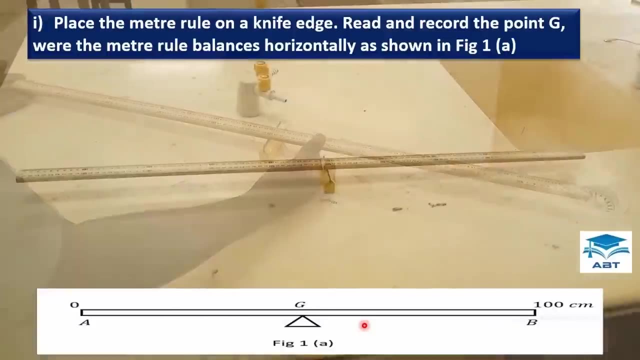 With the customized meter rule model, the outside of the motor routinely Y-axis, and this allows the meter to get neither this one nor that one. As the speed increases, both LEDs'll turn black and your left hand will simply shut up. Apply a hand to adjust. 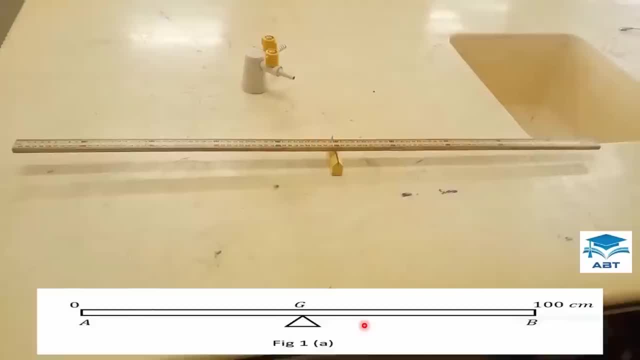 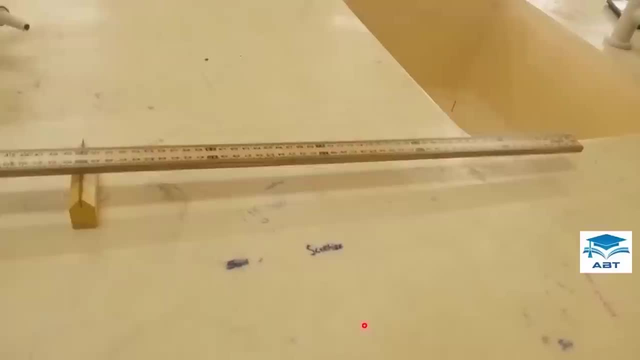 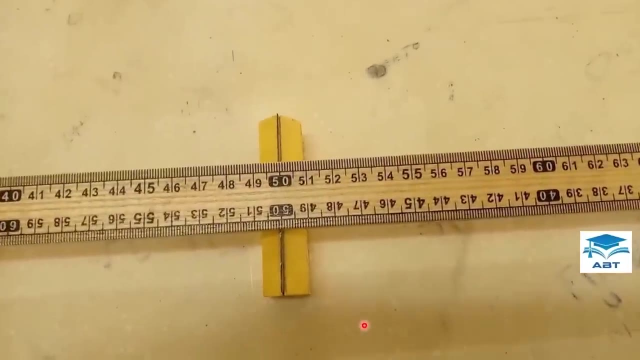 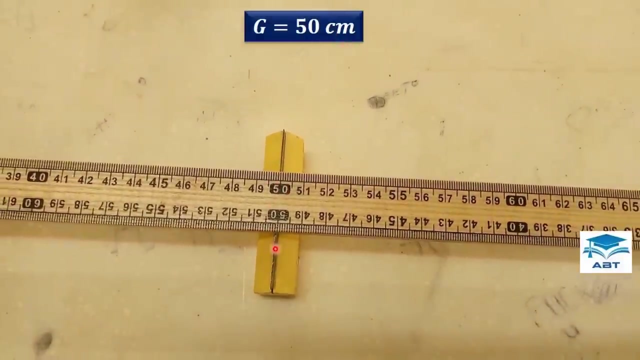 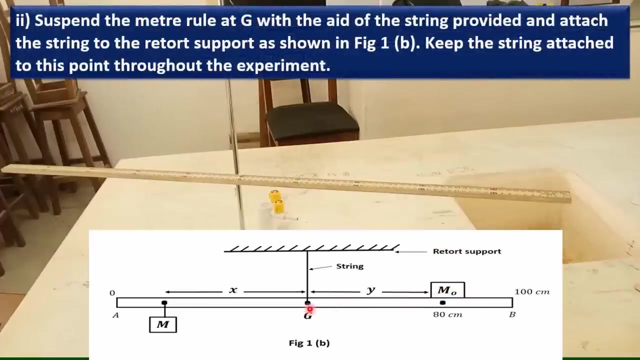 Try your left snowpack. Try to stay in the center. The point G is 50cm. Find the meter rule at G with the aid of the strength provided and attach the strength to the rate of support as shown in this diagram. We are going to keep the strength attached to this point throughout the experiment. 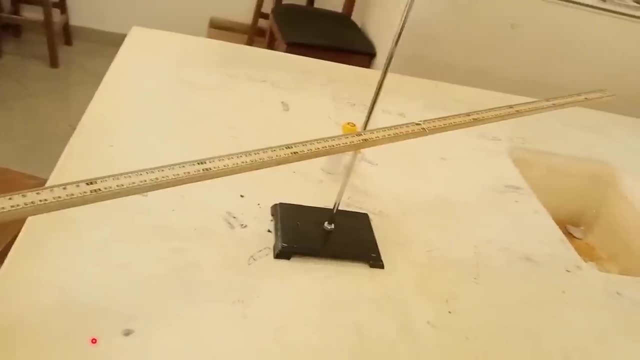 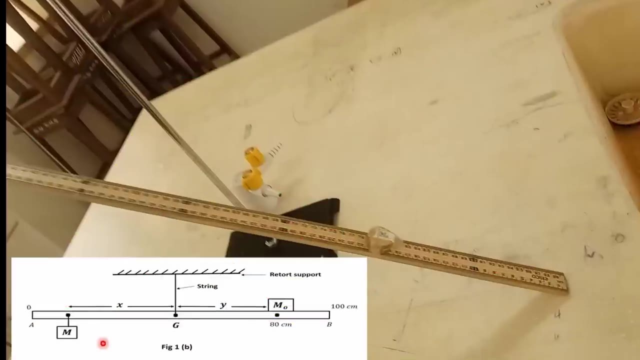 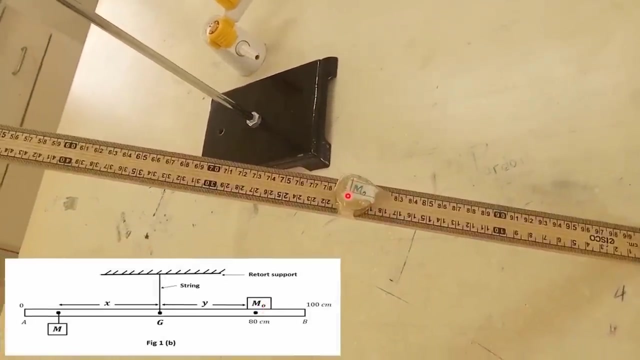 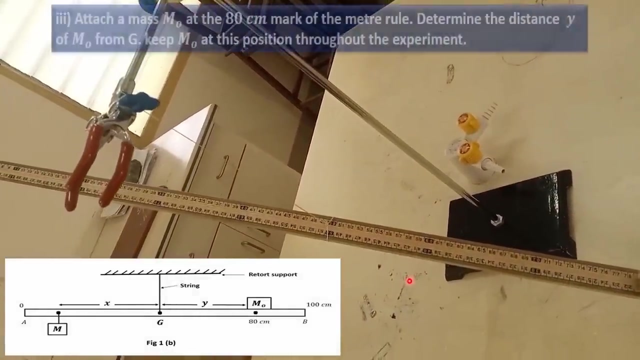 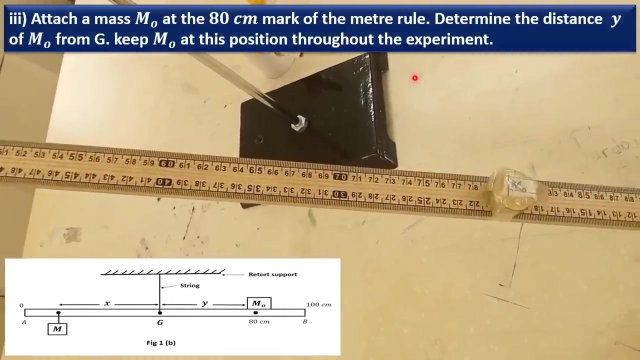 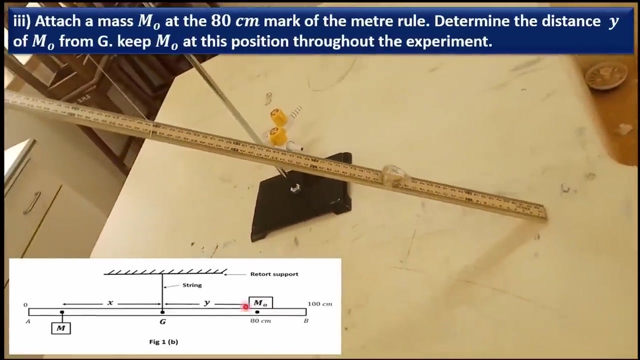 Another mass with a mass covered and M0 written on it have been provided. We are to fix that mass at the 80cm mark, measuring from this direction With the aid of a sellotape, And also determine the distance Y between M0 and G. 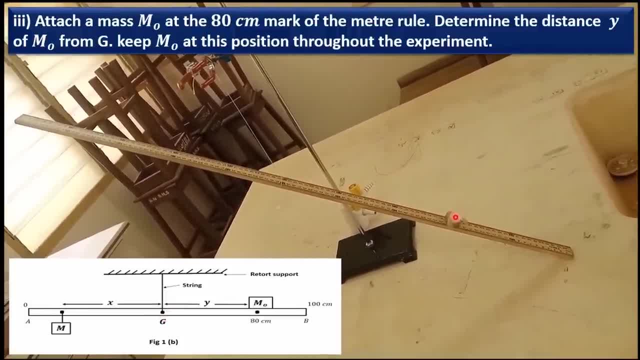 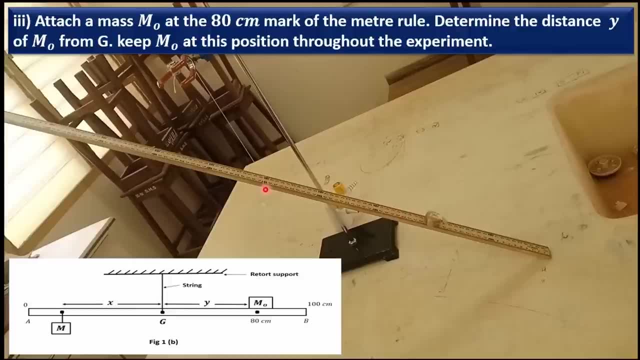 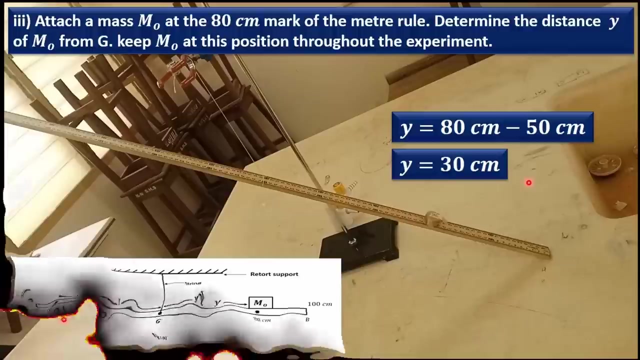 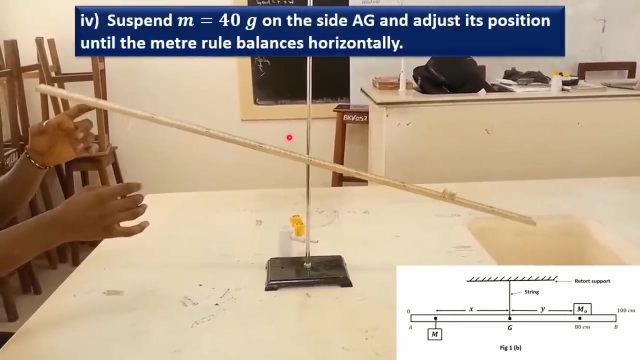 M0 is at 80cm And G is at 50cm, So the difference will give us Y, That is, Y is equal to 80cm minus 50cm, which is 30cm. We are going to suspend a mass of 40g on this side of the meter rule. 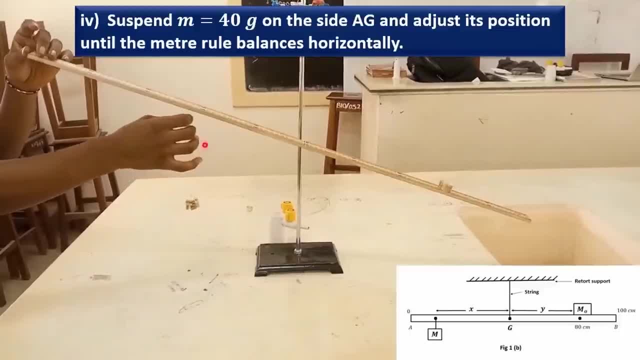 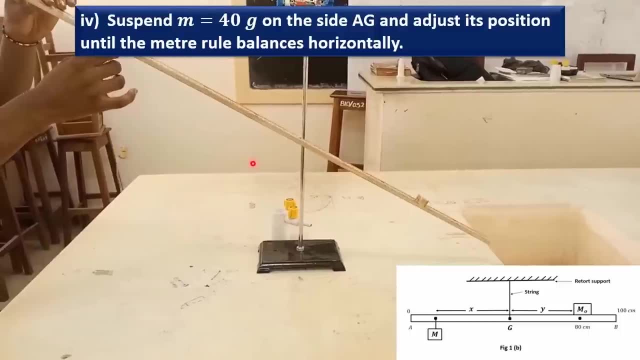 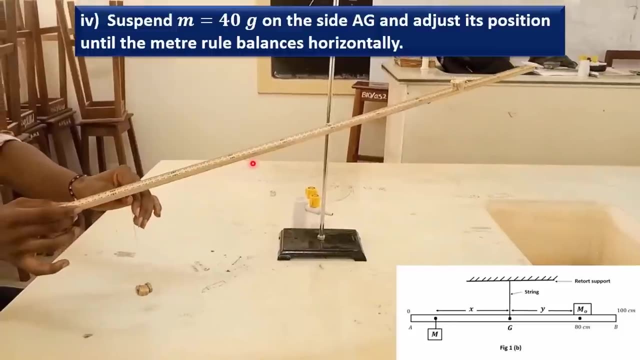 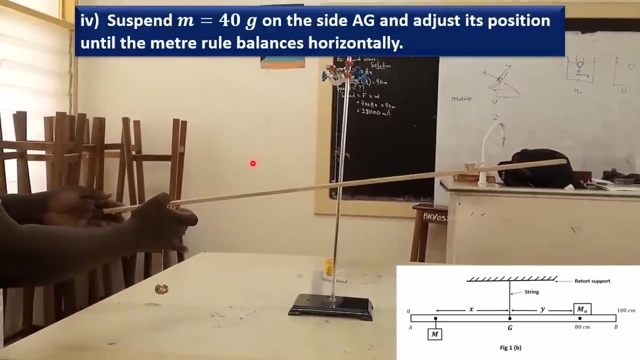 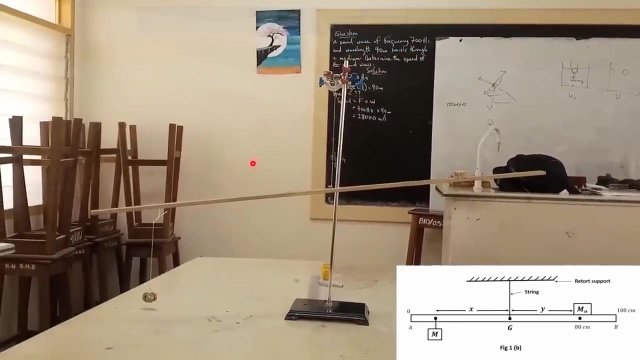 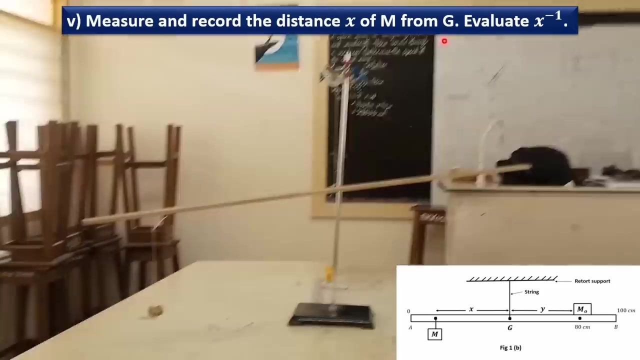 And adjust its position until the meter rule balances horizontal, The distance that you make from the center would be 22cm, But from that you're lost. Okay, So before we continue, Next exercise is a Rushu rep And we are going to measure and record the distance X of M from G. 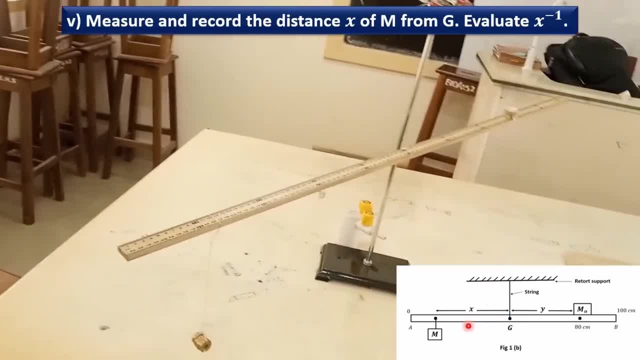 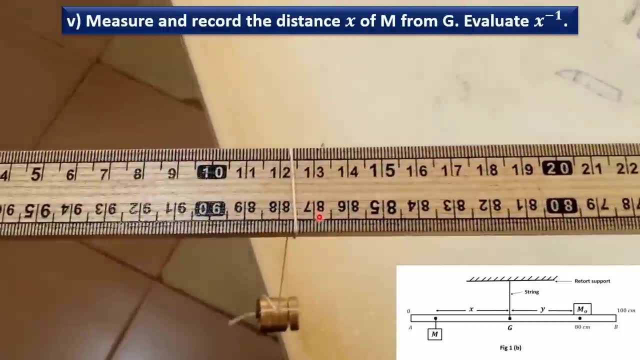 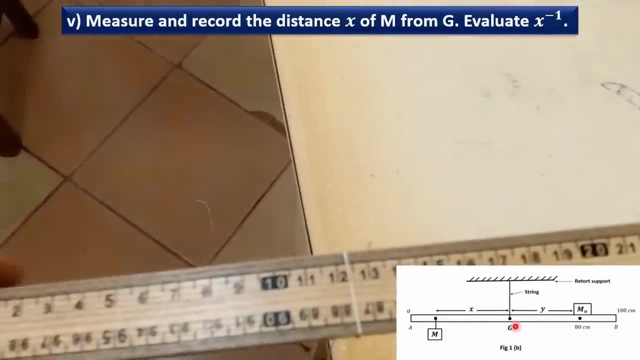 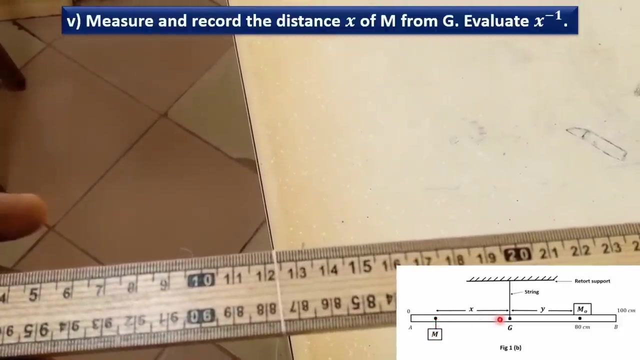 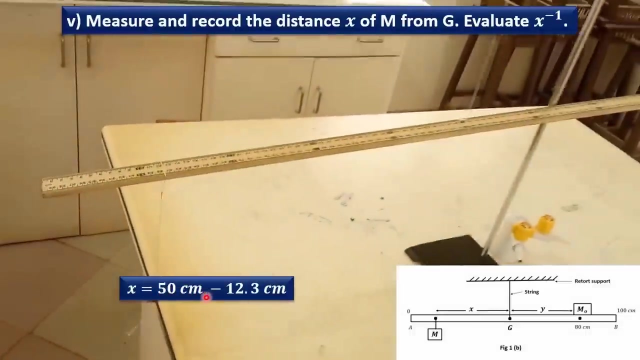 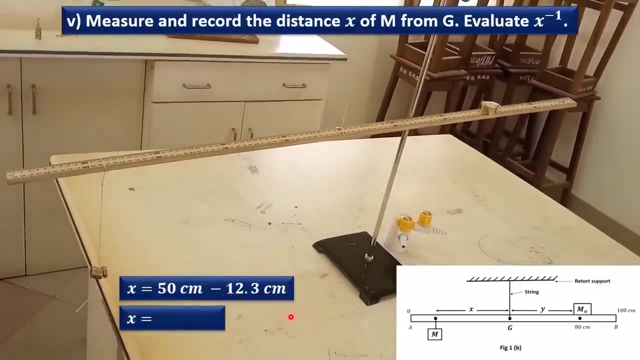 So G is 50 centimeters And M is 12.3 centimeters. So the difference between 50 centimeters and 12.3 centimeters is X. That is, X is equal to 50 centimeters minus 12.3 centimeters, which will give us 37.7 centimeters. 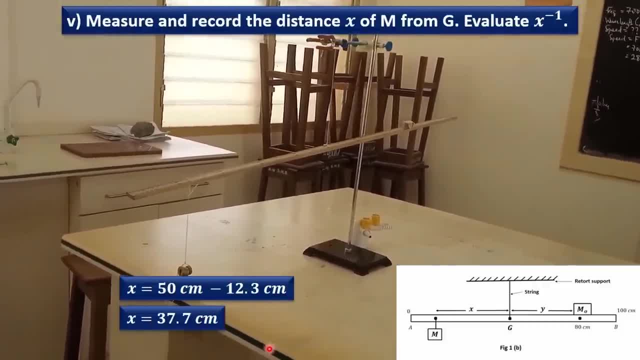 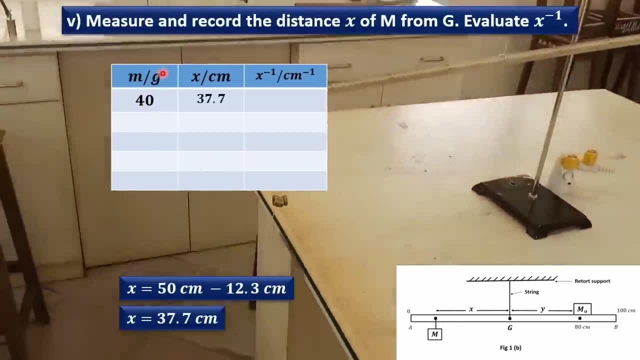 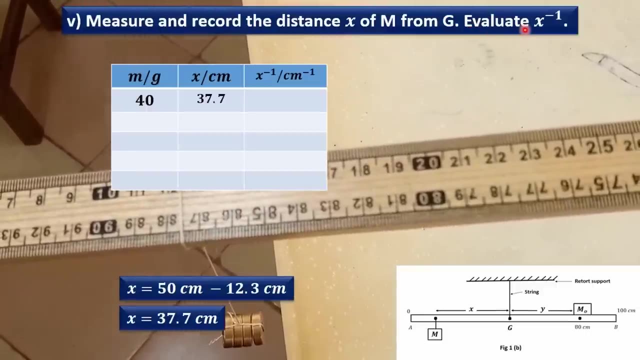 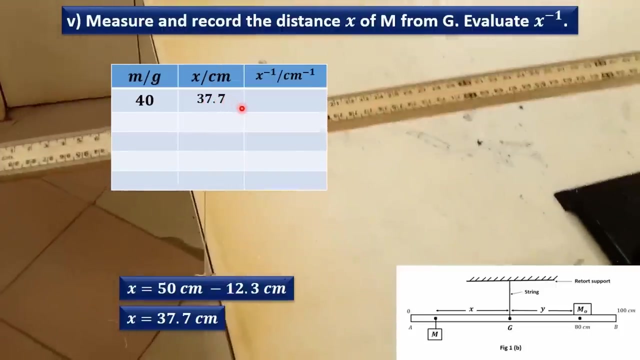 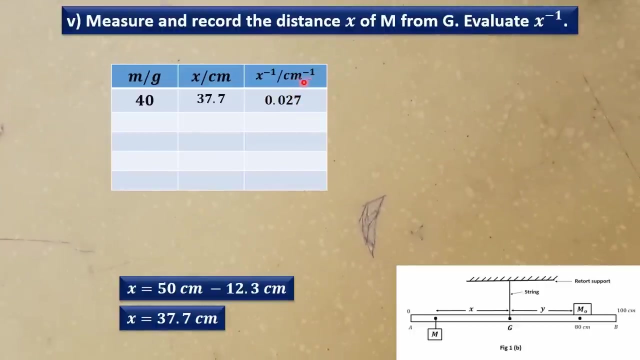 So the mass is 40 grams, X is 37.7 centimeters And we are going to evaluate X inverse. That is 1 divided by 37.7, which is 0.027.. That is 1 divided by 37.7, which is 0.027 per centimeters. 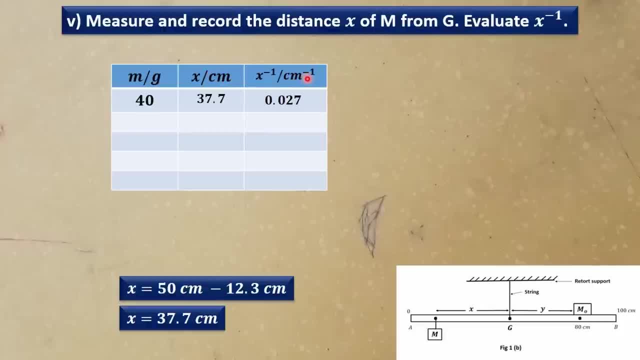 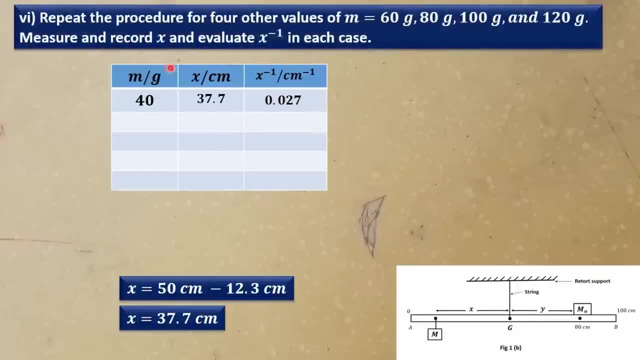 1 divided by centimeters is per centimeter, So that will be the unit over here. We are going to repeat the procedure for four other values. of M is equal to 60 grams, 80 grams, 100 grams and 120 grams. 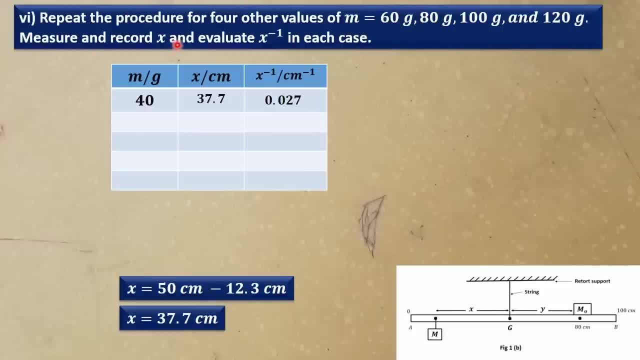 And we are going to measure and record X And evaluate X inverse in each case. So we change the mass to 60 grams, balance the meter row horizontally, determine X, find X inverse, Repeat the same thing for mass of 80.. 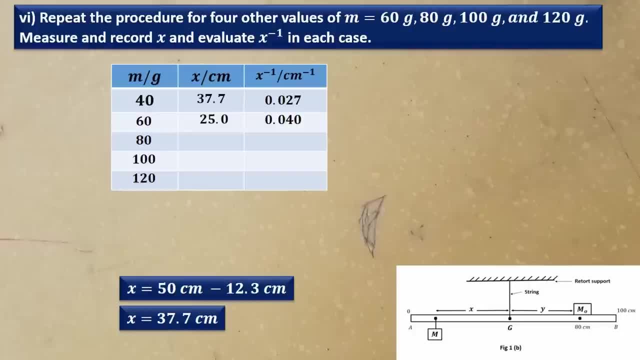 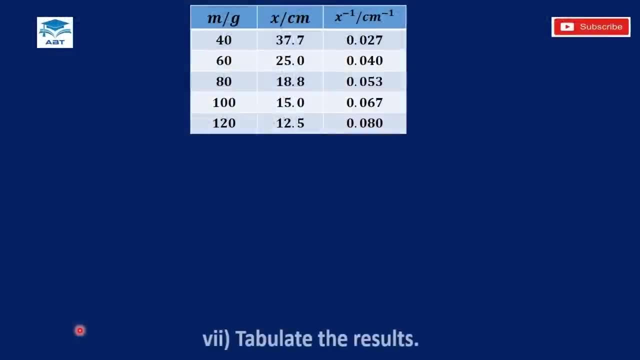 80 grams, 100 grams, 120 grams, and then tabulate the results. We are going to plot a graph of M on the vertical axis in the inverter graph on X, inverse on the horizontal axis, starting both axis from the origin 0, 0.. 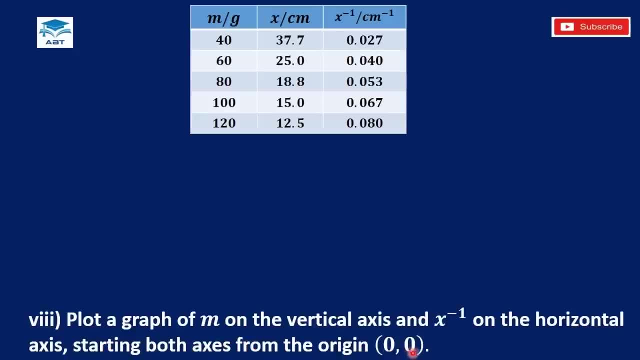 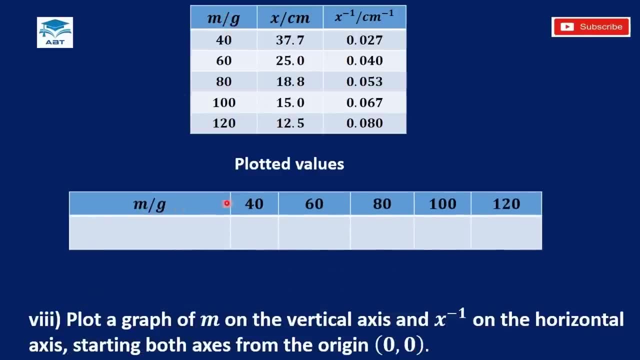 Awesome, So we can plot the scale: It's actually 0.027.. Alright, So we need the values of m, that is, 40,, 60,, 80,, 100 and 120 grams, And we also need the values of x inverse. 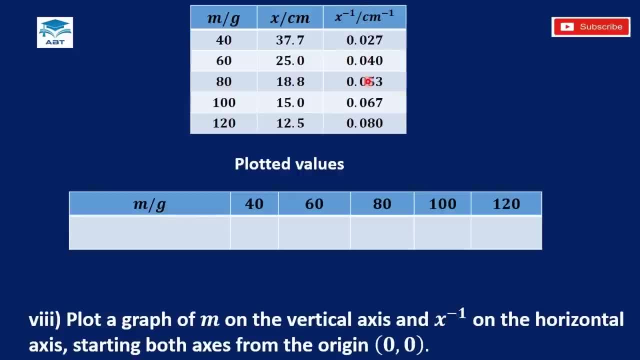 By looking at the values of x inverse. it will be difficult to plot the decimals, So we will convert them to standard form. We will move this point 1, 2, 3 to the right. So we have 27 over here times 10 exponent negative 3 in standard form. 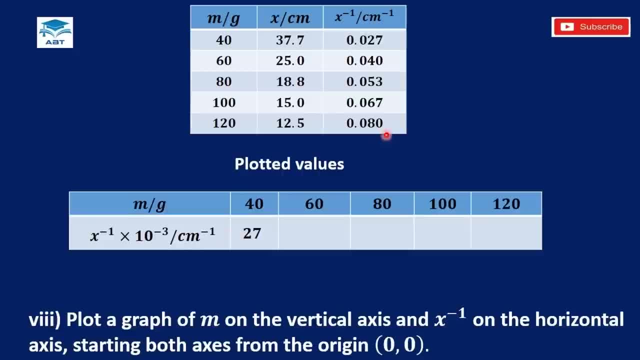 And the unit is per centimeters. So we move this one to 1,, 2,, 3 and up 40,, also times 10, exponent negative 3 per centimeters. So the next one will be 50 theory, the next one 67, and the last one is 80,, all times. 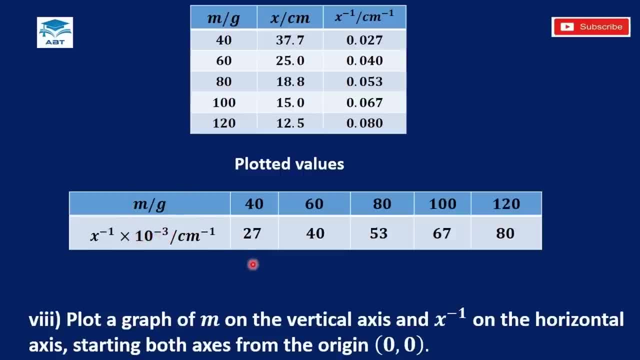 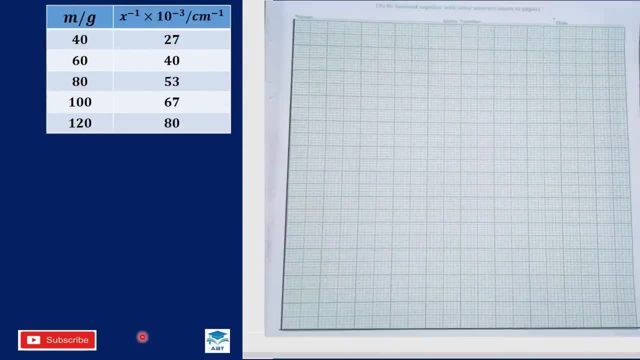 10 exponent negative 3 in standard form. So we draw the vertical and horizontal axis. Alright, Alright, We are plotting a graph of mass on the vertical axis and x inverse on the horizontal axis. So we choose a scale. We are going to choose a scale of 2cm x 10g on M axis. 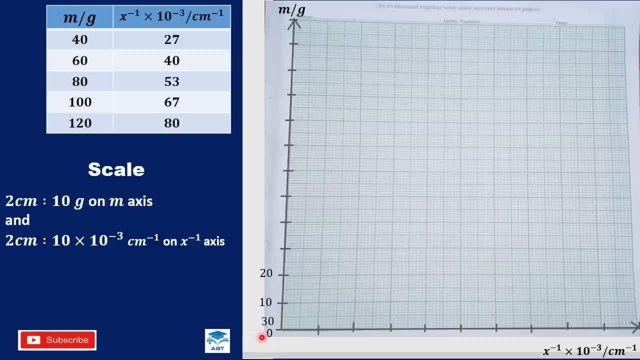 So we start from 0, 10,, 20,, 30,, 40 and so on. On x, inverse axis 2, we choose a scale of 2cm, representing 10 x 10-3 cm. So we start from 0,, 10,, 20,, 30 and so on. 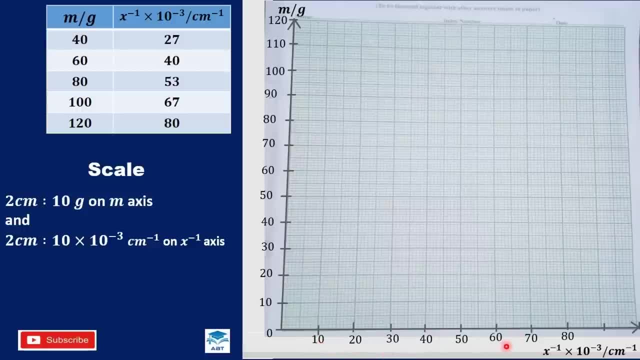 Remember these values are in standard form, So each value will be multiplied by 10-3.. Each box has 10 divisions. 10 divided by 10 is 1.. So each small box is equal to 1.. For the first point, we have 40 on the vertical axis and 27 on the horizontal axis. 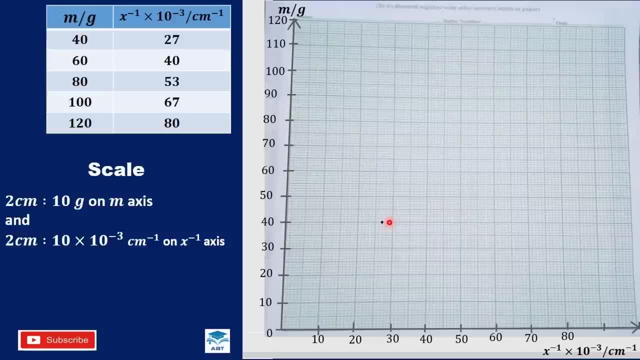 This is 20.. We have 7 more boxes or 27.. The next point: we have 60 on the vertical axis and 40 on the horizontal axis. meeting here. The next one: 80 on the vertical axis, 53 on the horizontal axis. 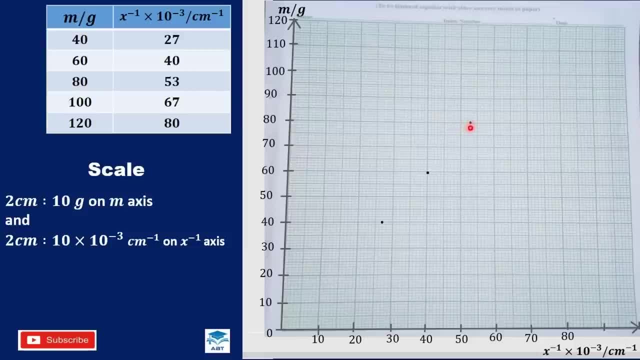 This is 50. We count 3 more boxes to the right and we have the point here. The next one: 100 on the vertical axis and 67 on the horizontal axis. This is 60.. We count 7 more boxes to the right and we have the point here. 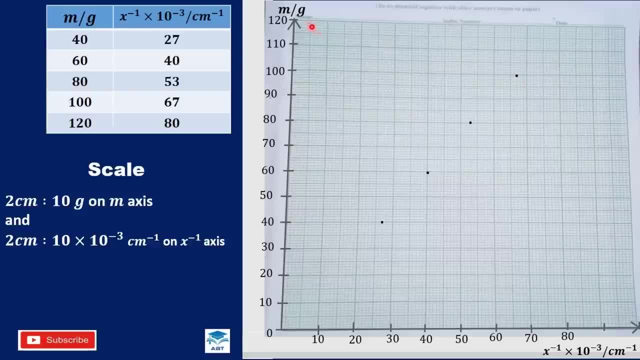 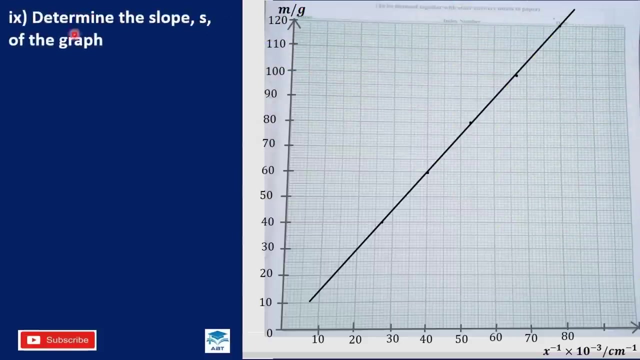 The last one. we have 120 grams on the vertical axis and 80 per cm on the horizontal axis meeting here. So we draw the line of best fit. We are going to determine the slope S of the graph. So for the slope we draw a horizontal and a vertical line. 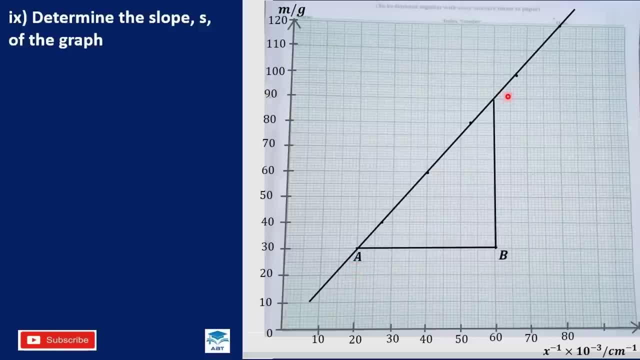 We name here A, here B and here C. The slope is change in BZ divided by change in BZ. For change in BC, we have 90 minus 30. And the unit on the vertical axis is grams. For change in AB, we have 60 minus 20.. 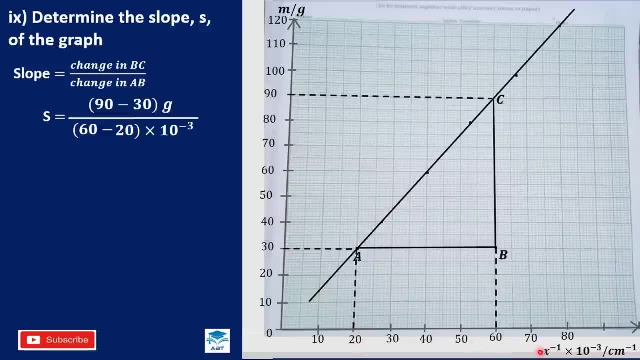 Remember times 10 is negative 3 on the horizontal axis And the unit is per cm. So 90 minus 30 is 60 grams And 60 minus 20 is 40. Remember times 10 is negative 3.. 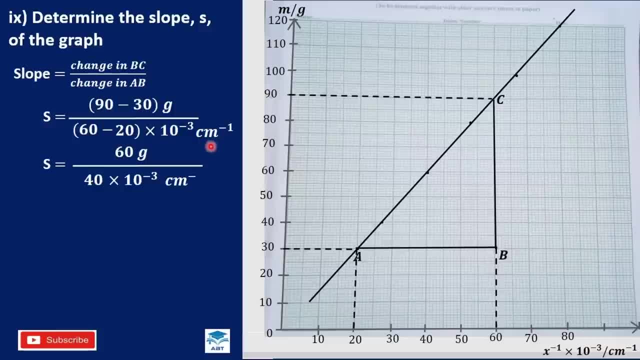 On the horizontal axis And the unit is per cm. 40 times 10 is 0.04.. And we are going to divide 60 by 0.04.. Which will give us 1500.. 1500 grams at the numerator. 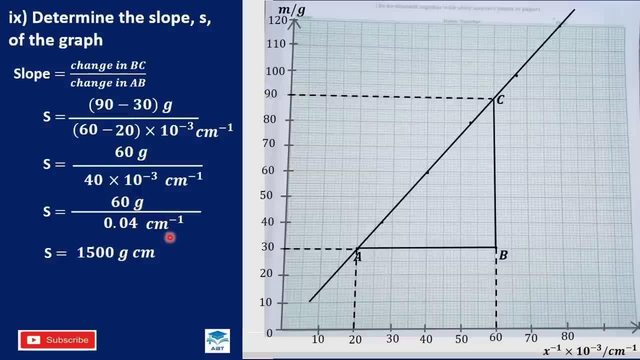 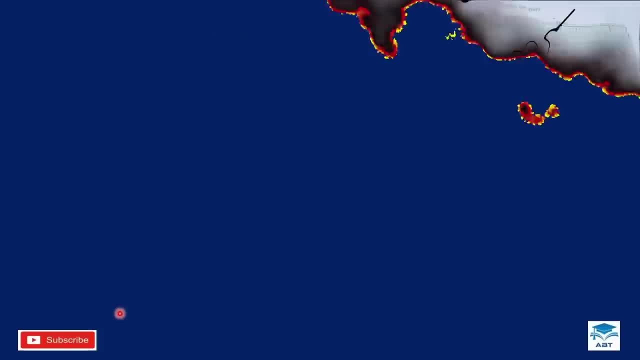 And when we reciprocate per cm, we have cm. So the unit is grams cm. Given that S is equal to Y times M0.. Determine M0.. We have S is equal to Y times M0.. So we divide both sides by Y. 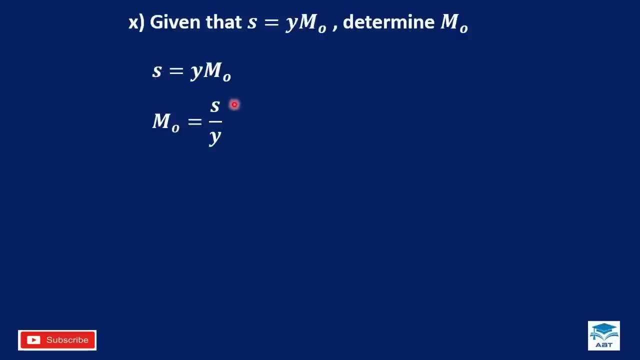 And we have: M0 is equal to S divided by Y, But the slope is 1500 grams cm And Y is 30 cm. So we divide 1500 by 30. And we have 50 cm. So we cancel out.